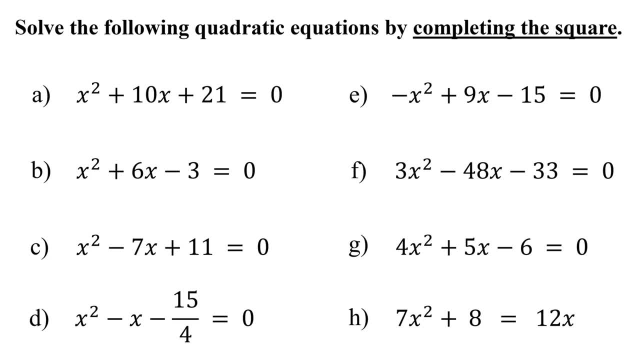 In this video, you will learn how to solve quadratic equations using the Completing the Square method. We will work through different examples, starting with equations with a leading coefficient of 1, and then those with a leading coefficient different from 1.. Let's get started. 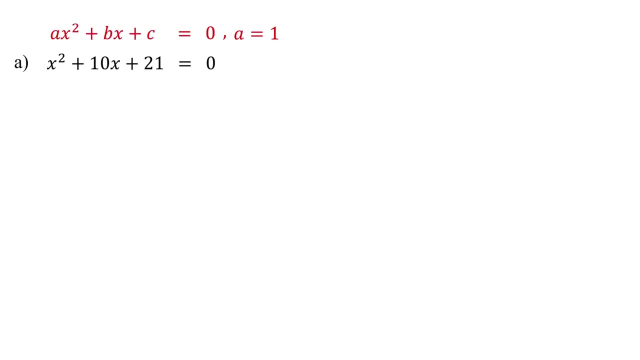 If a quadratic equation is given in standard form with a leading coefficient of 1,, our first step is to move the constant term to the right side of the equation. In this example, we can do this by subtracting 21 from both sides of the equation. 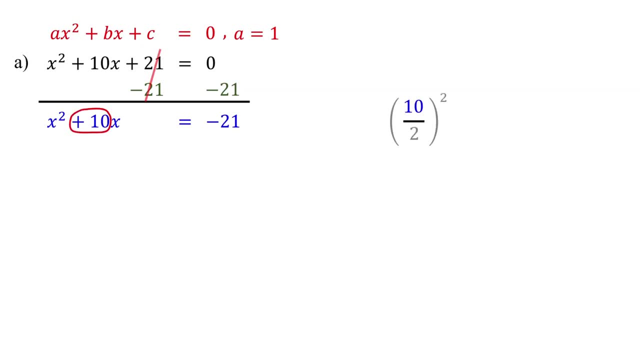 Next, we find half of the coefficient of x and square it. Half of 10 is 5, and 5 squared is 25, right, Then we add this value to both sides of the equation. This addition transforms the expression on the left side into a perfect square trinomial. 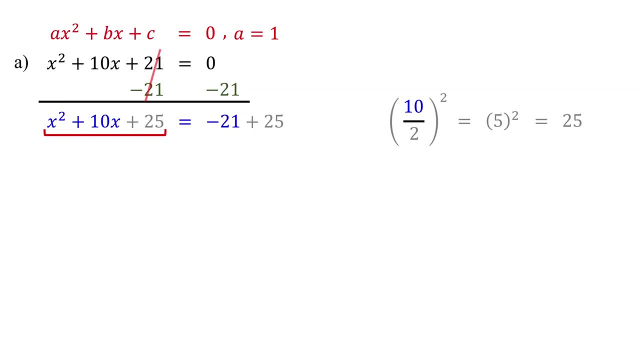 Our next step is to rewrite this trinomial as a binomial square, which will be x plus 5 squared. The number in the binomial always corresponds to half of the coefficient of 1.. Next, we will add the coefficient of x in the perfect square trinomial, which is 5 in this case. 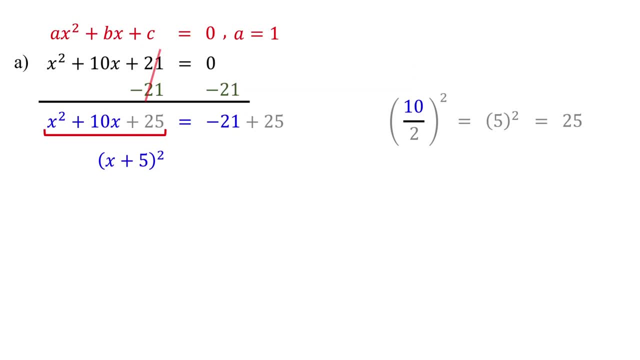 Notice that by adding a specific number, we complete the square. This is why the method is named Completing the Square. On the right side, negative 21 plus 25 equals 4.. Next we take the square root of both sides According to the square root property. 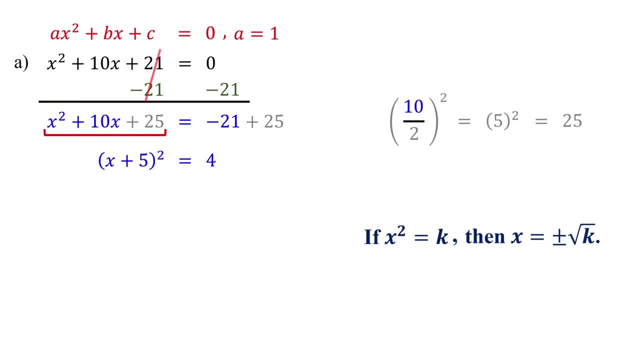 if x squared equals a real number k, then x equals plus or minus the square root of k. Not so easily is down, but we eat. x squared is more or less a real number k. So we have: x plus 5 equals plus or minus the square root of 4.. 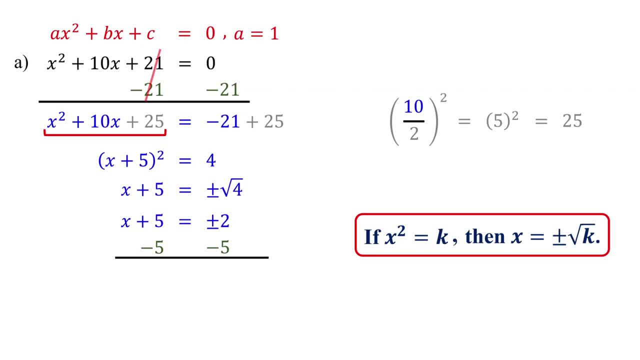 The square root of 4 is 2, right. Finally, we solve for x by subtracting 5 from both sides. These cancel out and we get x equals negative, 5 plus or minus 2.. This is the same as x equals. 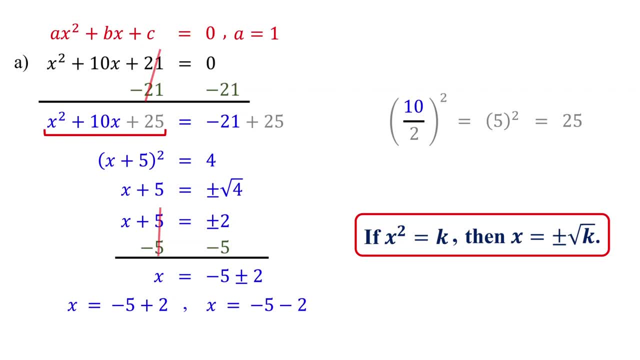 negative 5 plus 2, or x equals negative 5 minus 2.. Therefore, the solutions are: x equals negative 3, or x is negative 3 or minus 3. equals negative seven. We can check our solutions by substituting them back into the original. 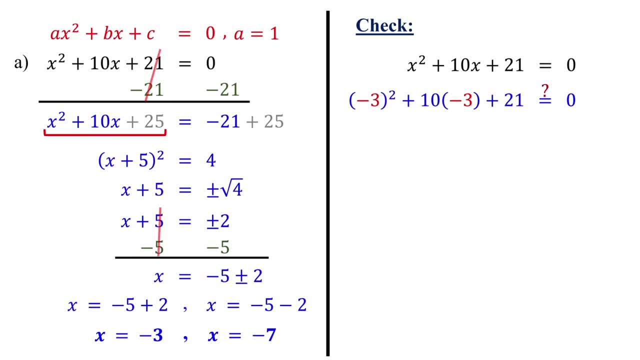 equation: Substituting negative three: negative three squared is nine and ten times negative three is negative. thirty Nine minus thirty is negative twenty-one and this equals zero right. Similarly, substituting negative seven: negative seven squared is forty-nine and ten times. 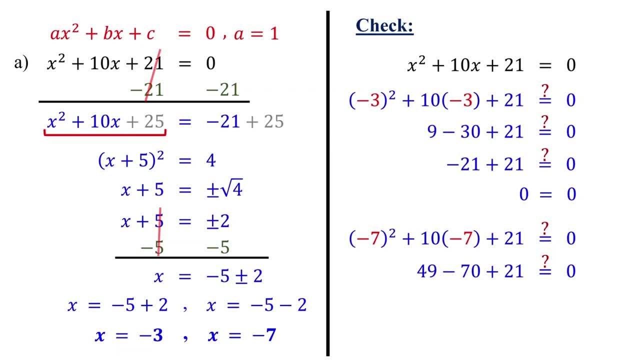 negative seven is negative seventy. Forty-nine minus seventy is negative twenty-one, and this equals zero. As you can see, both negative three and negative seven are valid solutions. Let's discuss why, in some cases, we need to use the completing the square method instead of the. 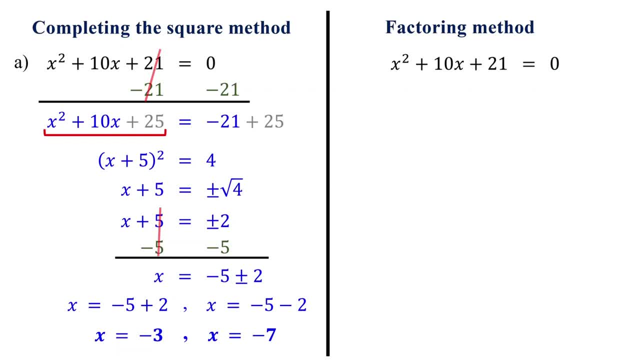 factoring method. This quadratic equation can be easily solved by factoring, as it is simple to find two numbers that multiply to give twenty-one and add up to ten. These numbers are three and seven right. Three multiplied by seven equals twenty-one. 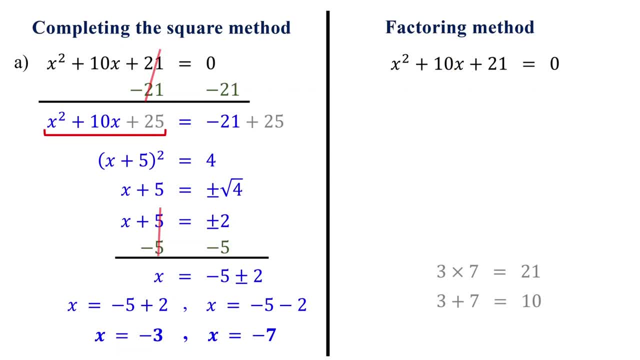 and three plus seven equals ten. So when we factor this quadratic equation, it becomes x plus three times x plus seven, which equals zero. Now, setting each factor equal to zero and solving for x gives us the solutions. As you can see, the factoring method is easier and faster for this example, right? However, 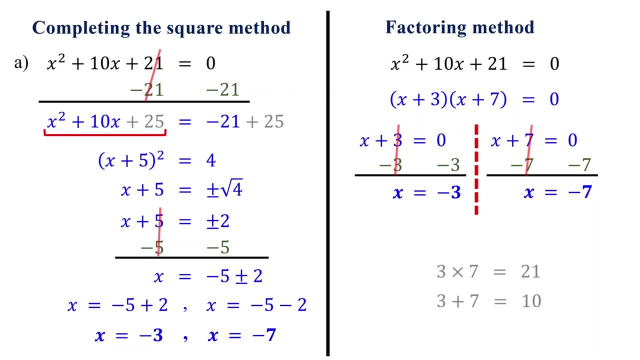 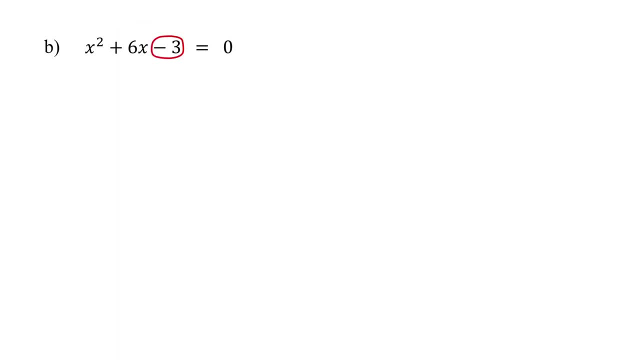 the quadratic trinomial can be factored, But all can be solved by completing the square. For instance, in the next example, it is difficult to find two numbers that multiply to give negative three and add up to six. Can you find these numbers? It is difficult, right? So this quadratic? 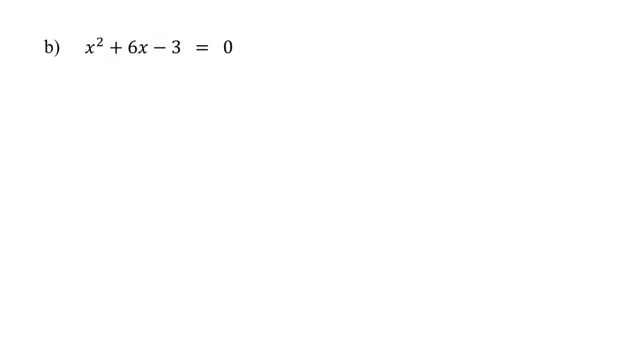 equation is challenging to factor. However, it can be easily solved using the completing the square method. Since this quadratic equation is also in standard form with a leading coefficient of one, our first step is to move the constant term to the right side of the equation. Next, 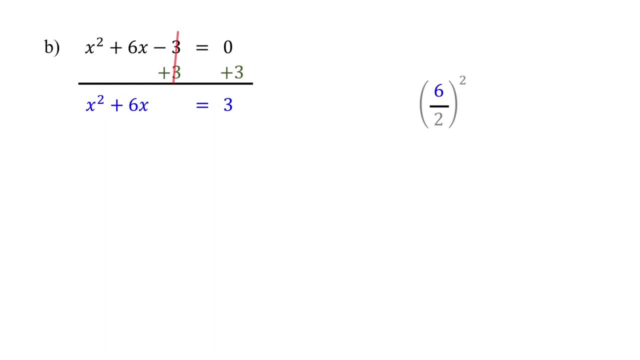 find half of the coefficient of x and square it. Half of six is three, and three squared equals nine. Then add this value to both sides of the equation. This addition transforms the expression on the left side into a perfect square trinomial. Our next step is to rewrite this trinomial as a. 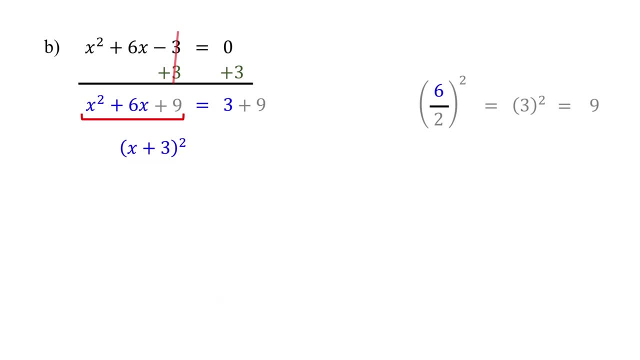 binomial square which will be x plus three squared. Remember, the number in the binomial always corresponds to half of the coefficient of x. in the perfect square trinomial On the right side, three plus nine equals twelve. Next take the square root of both sides. The square root of twelve simplifies to two times. 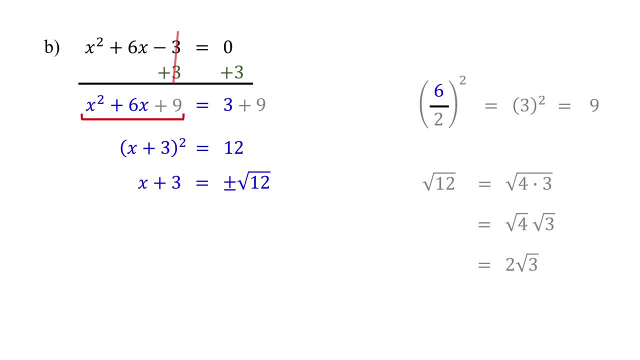 the square root of three. right, So we have x plus three equals plus or minus two root three. Finally, solve for x by subtracting three from both sides. This gives us x equals negative three plus or minus two root three. You can leave your solution. 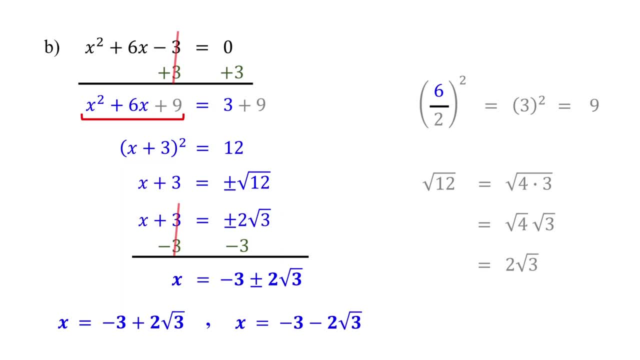 as it is or write the two solutions separately. Both are possible ways of writing the solutions. Let's work on more examples that are difficult to solve with factoring but possible with the completing the square method. By the way, you can solve any quadratic trinomial using the completing. 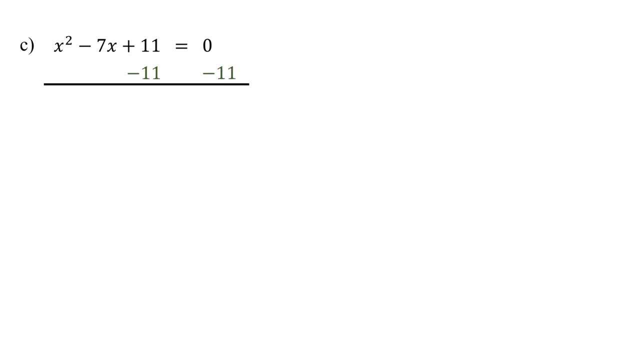 the square method. First, move the constant term to the right side of the equation. Next, find half of the coefficient of x and square it. Since negative seven does not divide evenly by two, we leave it as a fraction. Negative seven squared is forty-nine and two squared is four. 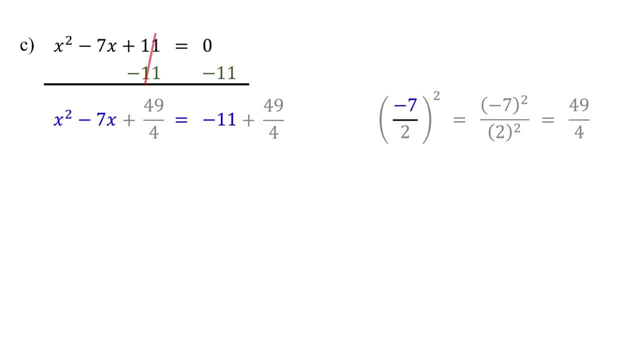 Then add this value to both sides of the equation. Now write this perfect square trinomial as a binomial square. This number is half of the coefficient of x in the perfect square trinomial On the right side. add negative eleven and forty-nine over four. 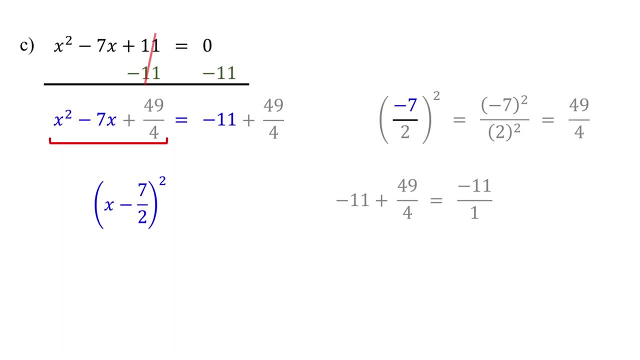 Negative eleven is the same as negative eleven over one right To get a common denominator. multiply it by four over four. Negative eleven times four is negative forty-four and one times four is four. Now add the numerators, which equals five. 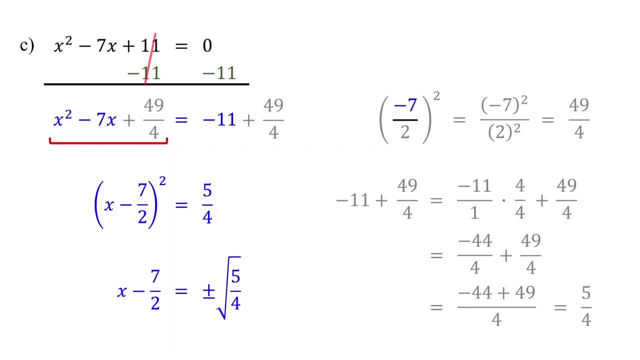 The next step is to take the square root of both sides. The square root of five over four simplifies to the square root of five over two. Finally, solve for x by adding seven halves to both sides of the equation. You can leave your solution as it is or write the two solutions separately. 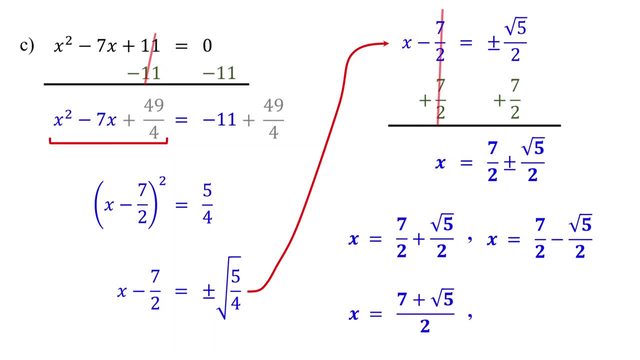 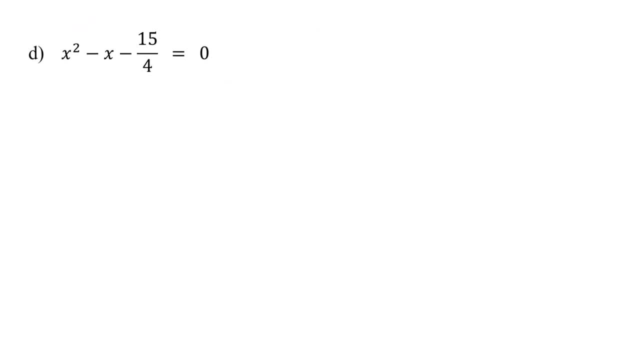 In fact, because the denominators are the same, you can combine the numerators. All of these are acceptable ways of writing the solutions. This one is for you. Please pause the video and give it a try. First, move the constant term to the right side of the equation. 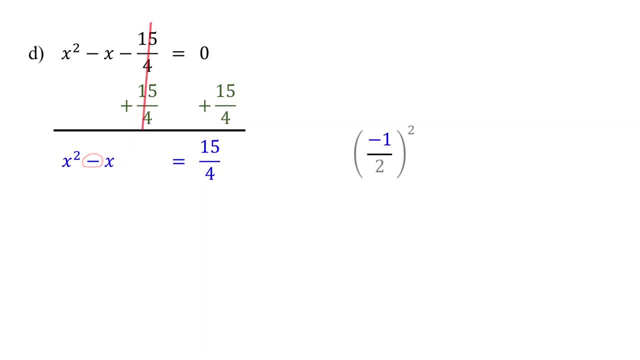 Next, find half of the coefficient of x and square it Negative. one squared is one and two squared is four. Then add this value to both sides of the equation. Now write this perfect square trinomial as a binomial square. 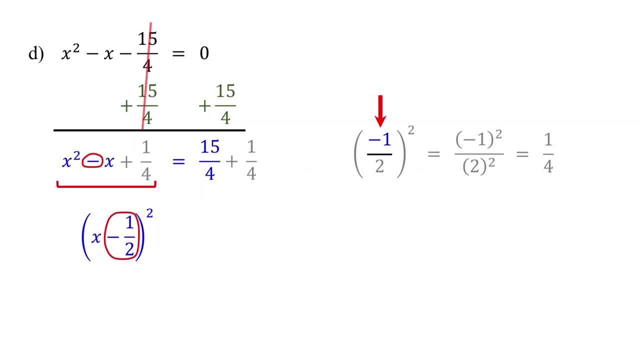 This number is half of the coefficient of x in the perfect square trinomial On the right side. add the fractions. Since they have a common denominator, simply add the numerators. Next, take the square root of both sides. The square root of four is two. 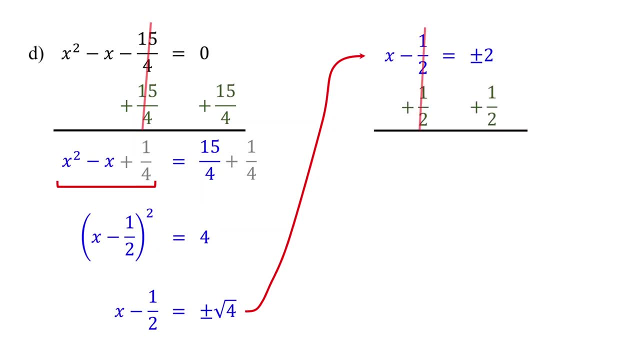 Then solve for x by adding one half to both sides of the equation. This is the same as x equals one half plus two or x equals one half minus two. Therefore, the solutions are: x equals five halves or negative three halves. 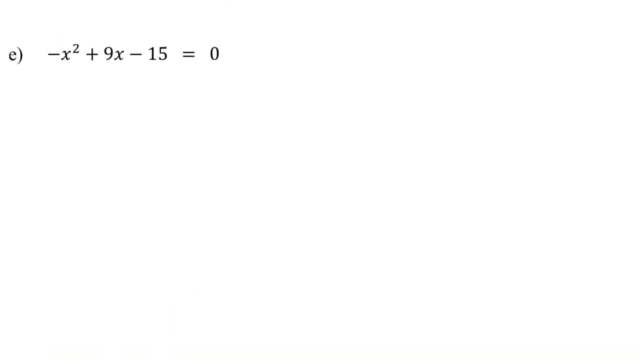 Now let's work on quadratic equations with a leading coefficient different from one. To complete the square, we need to add one half to both sides of the equation. To complete the square, the leading coefficient must be one. So when the leading coefficient is different from one, our initial step is to make it one. 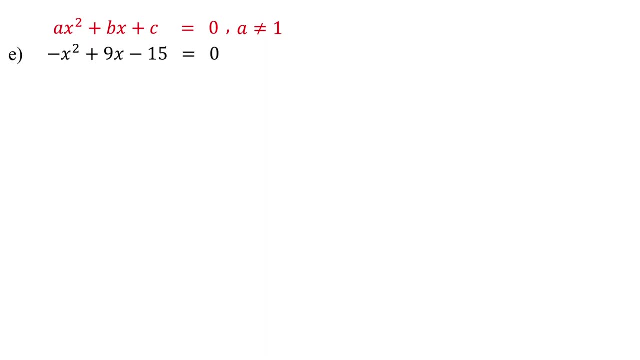 We do this by dividing each term in the equation by the leading coefficient itself. In this case, the leading coefficient is negative one, So we divide each term in the equation by negative one. As you can see, the leading coefficient is now one. 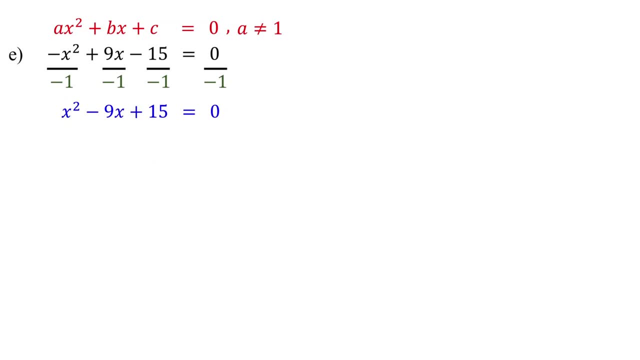 From this point forward, we follow the same steps as in the previous example: Move the constant term to the right side of the equation. Next find half of the coefficient of x and square it Negative. nine squared is eighty-one and two squared is four. 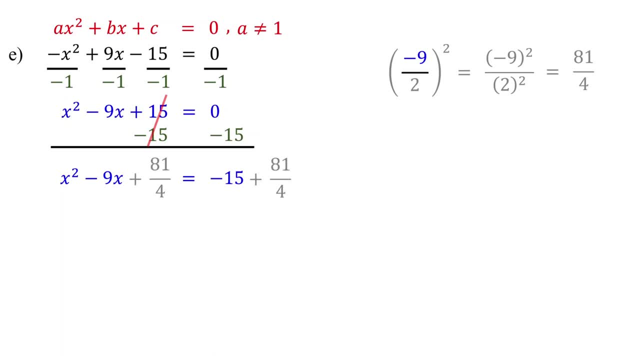 Then add this value to both sides of the equation. Now write this perfect square trinomial as a binomial square. Remember the number in the binomial is half of the coefficient of x in the perfect square trinomial. Now add this value to both sides of the equation. 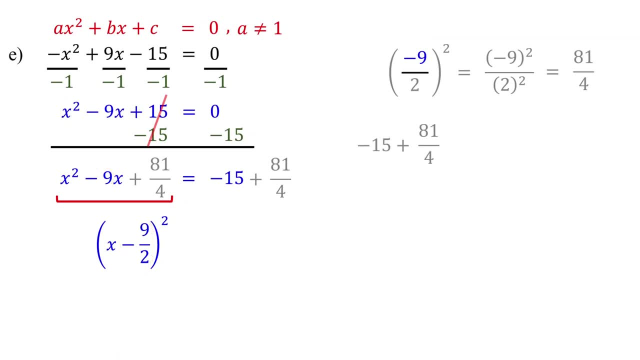 On the right side. add negative fifteen and eighty-one over four. Negative fifteen is the same as negative fifteen over one. right To get a common denominator. multiply it by four over four. Negative fifteen times four is negative sixty and one times four is four. 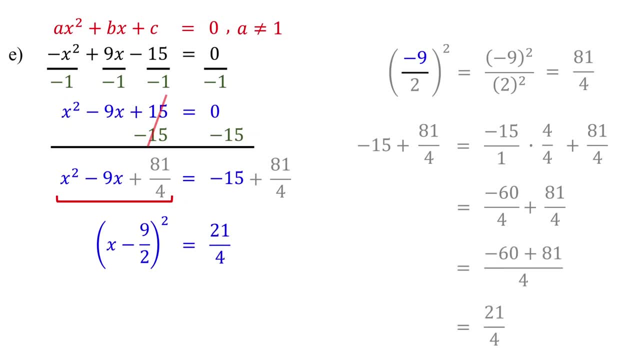 Now add the numerators, which equals twenty-one. Next take the square root of both sides. The square root of twenty-one over four is negative fifteen. The square root of twenty-one over four simplifies to the square root of twenty-one over two. 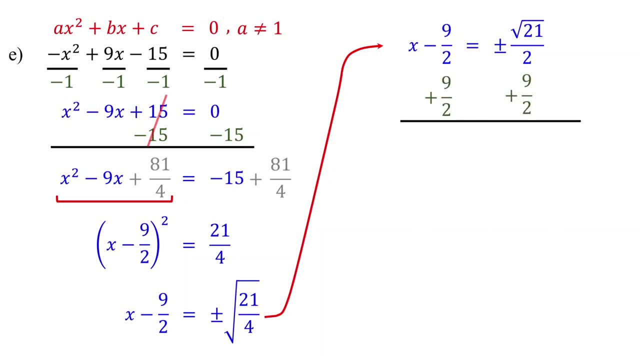 Finally solve for x by adding nine halves to both sides of the equation. You can leave your solution as it is, or write the two solutions separately, or combine the numerators, since the denominators are the same. If you have found this video helpful so far, please give it a thumbs up and consider subscribing. 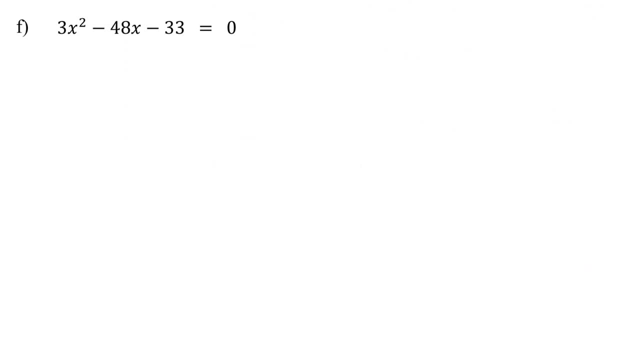 This one is for you. Please pause the video and give it a try. In this example the leading coefficient is three. So first divide each term in the equation by three to make the leading coefficient one. Then move the constant term to the right side of the equation. 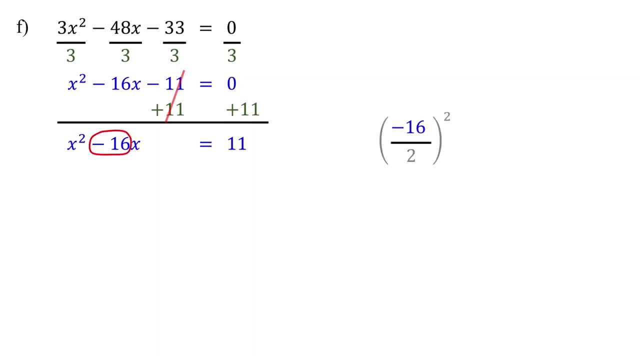 Next, find half of the coefficient of x and square it. Half of negative sixteen is negative eight, and negative eight squared equals sixty-four. Then add this value to both sides of the equation. Now write this perfect square root of twenty-one over four. 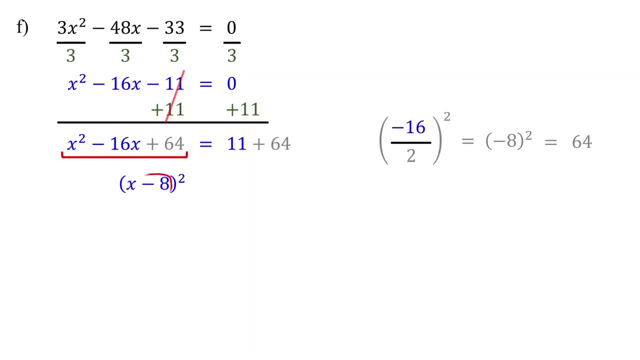 This is the perfect square trinomial. as a binomial square, This number is half of the coefficient of x. in the perfect square trinomial On the right side, eleven plus sixty-four equals seventy-five. Next take the square root of both sides. 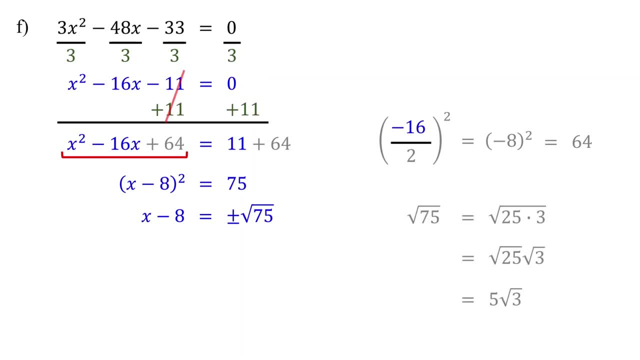 The square root of seventy-five simplifies to five times the square root of three. Then solve for x by adding eight to both sides of the equation. Therefore, these are the solutions. The next example is a bit more challenging. It involves many fractions in the process of solving, so please stay with me. 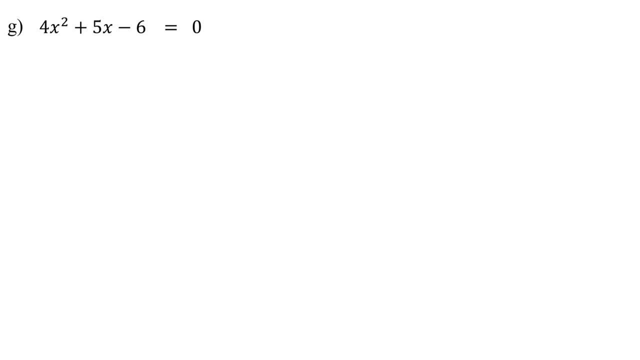 The leading coefficient is four. So first divide each term in the equation by four to make the leading coefficient one. Then move the constant term to the right side of the equation. Next find half of the coefficient of x and square it. 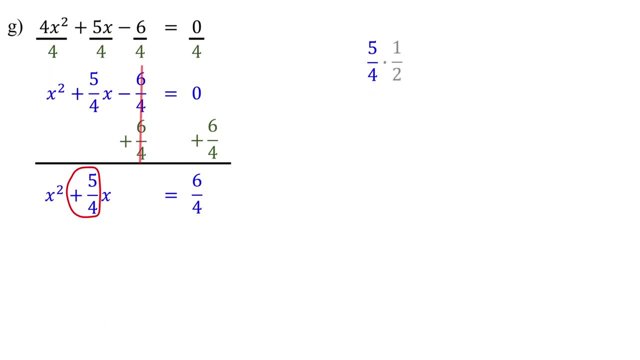 Dividing by two is the same thing as multiplying by one half. Five times one is five and four times two is eight. Five squared is twenty-five and eight squared is sixty-four. Then add this value to both sides of the equation. 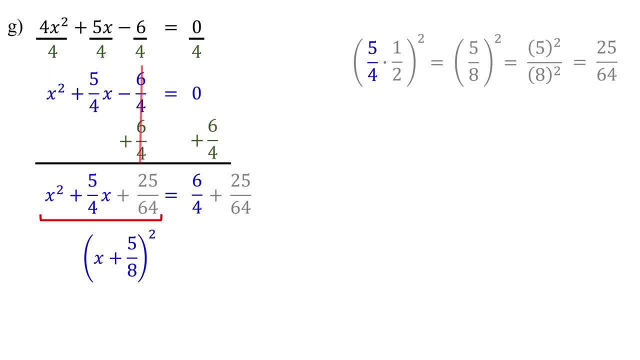 Next write this perfect square trinomial as a binomial square. This number is half of the coefficient of x in the perfect square trinomial On the right side. add the fractions To get a common denominator. multiply the first fraction by sixteen over sixteen. 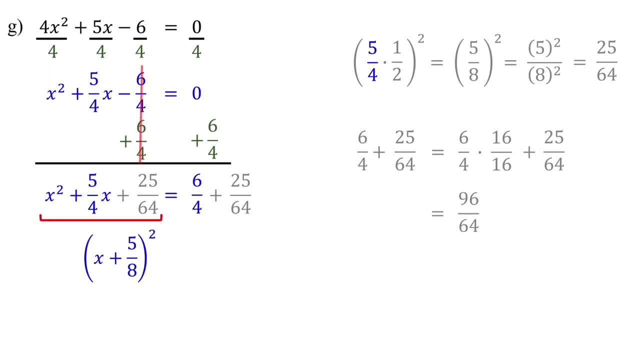 Six times sixteen is ninety-six, and four times sixteen is sixty-four. Now add the numerators, which equals one hundred and twenty-one. Next, take the square root of both sides: The square root of one hundred twenty-one is eleven and the square root of sixty-four is eight. right, 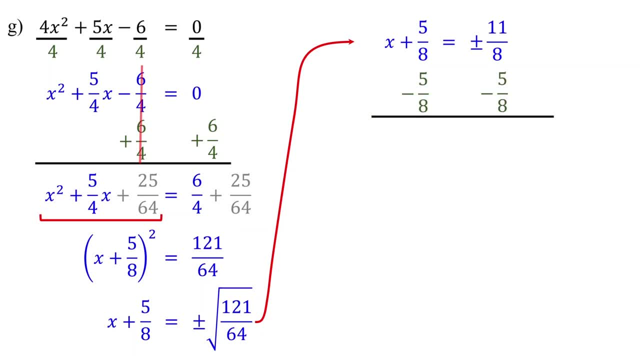 Finally, solve for x by subtracting five-eighths from both sides. One of the solutions is negative: five-eighths plus eleven-eighths. Add the numerators, since they have the same denominator. This simplifies to three-fourths. 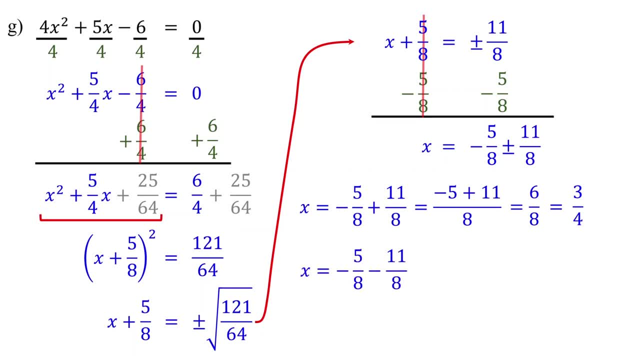 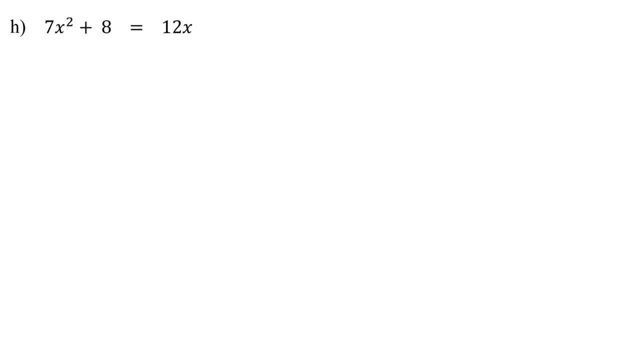 The other solution is negative. five-eighths minus eleven-eighths. This is equal to negative two. Therefore, these are the solutions. In the next example, the quadratic equation is not in standard form. What should be our first step In this case? the first step is to rewrite the quadratic equation in standard form. 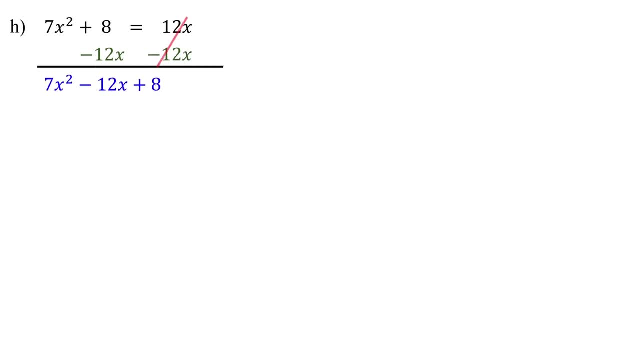 To do this, subtract twelve x from both sides of the equation. Next divide each term in the equation by seven to make the leading coefficient one. Then move the constant term to the right side of the equation. Next find half of the coefficient of x and square it. 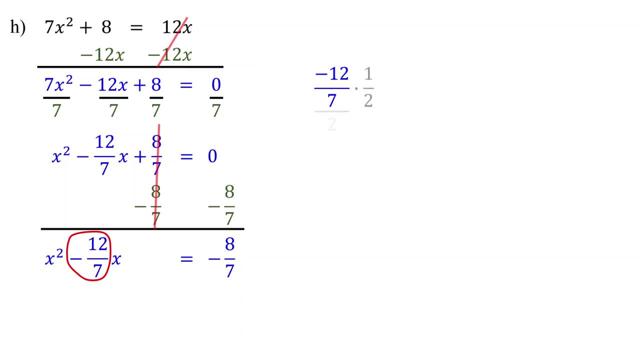 Remember, dividing by two is the same thing as multiplying by one-half. Simplify negative twelve and two to negative six, Leaving us with negative six over seven. Negative six squared is thirty-six and seven squared is forty-nine. Then add this value to both sides of the equation. 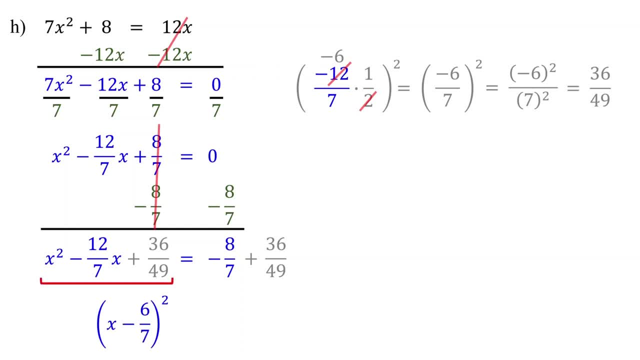 Next write this perfect square trinomial as a binomial square. This number is half of the coefficient of x in the perfect square trinomial On the right side. add the fractions To get a common denominator. multiply the first fraction by seven over seven.